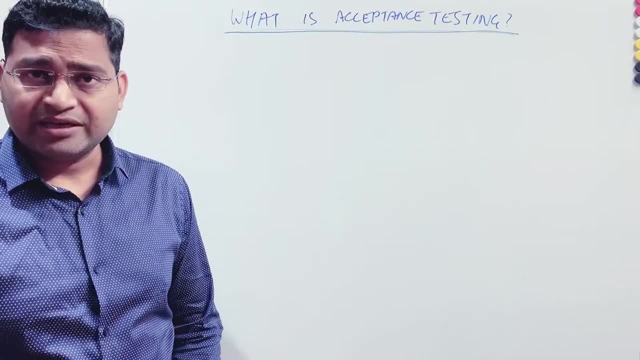 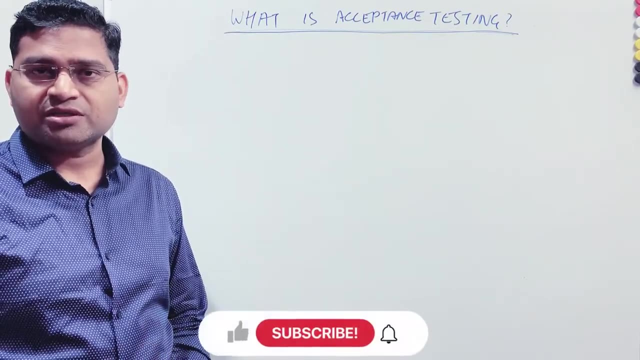 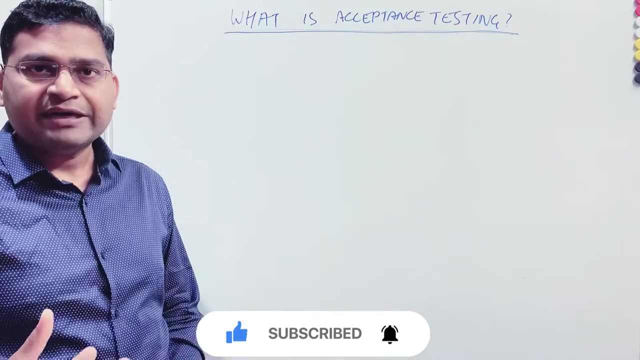 testing. Now to understand acceptance testing, I'll take an example here: how the customer provides the requirement, right? so there are some needs or customer requirements that are being explained to the team who is developing the software, and that's how the requirements come in picture, right? so 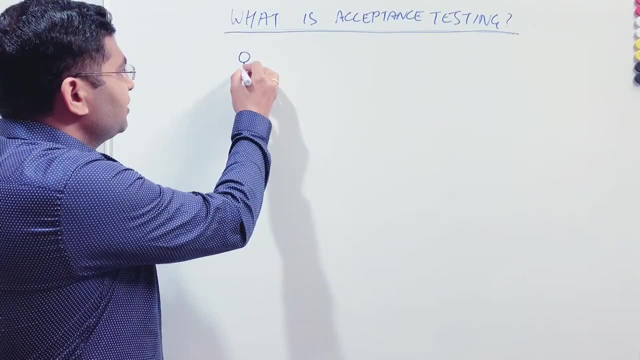 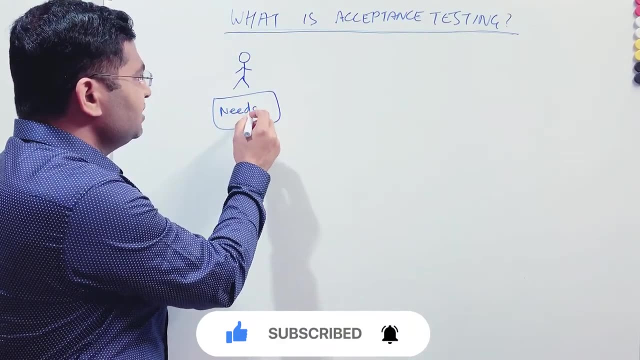 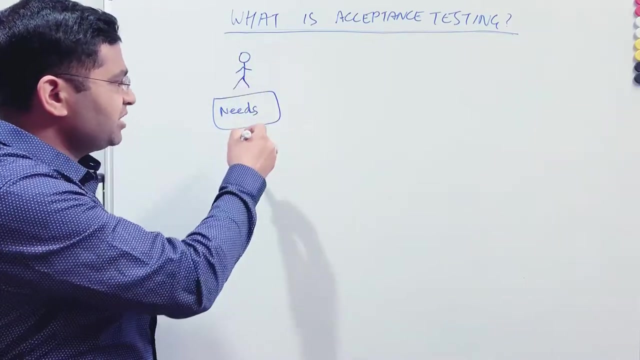 say, for example, there is a customer, okay, and he has certain requirements or needs, right, so what he actually actually needs. so he will explain that, or he will, you know, document that, that and he'll send those details, or he'll try to explain that these are my needs, in say for: 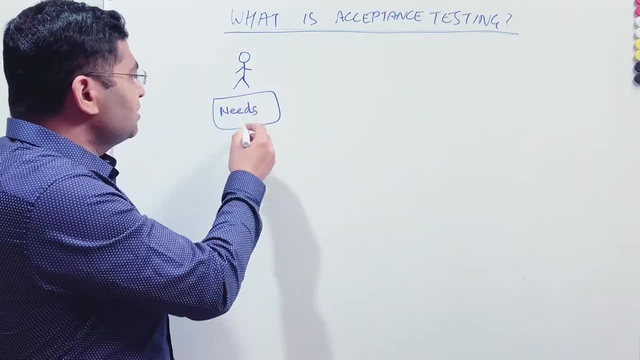 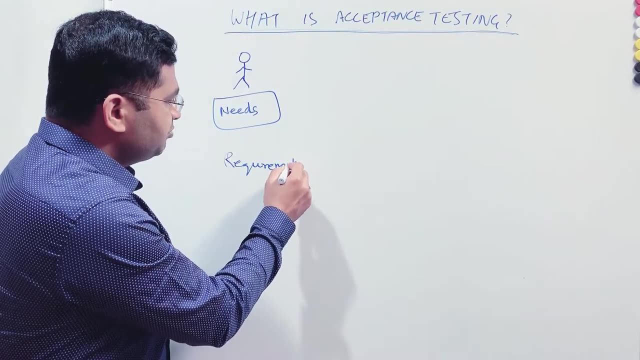 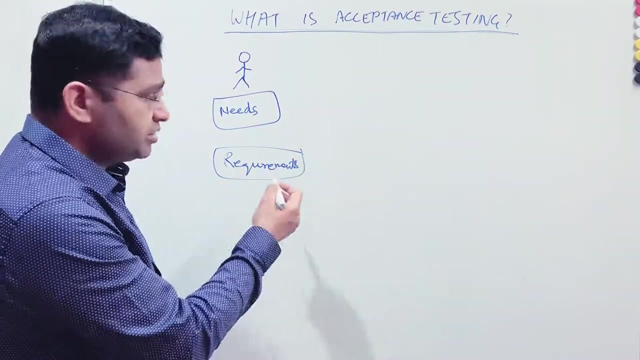 example, e-commerce website, and based on that needs, somebody will document those into requirements, right? so if it is, you know, waterfall approach, there will be big requirement documentations. otherwise, if it is agile or scrum, agile scrum, then it will be user stories. now how will the 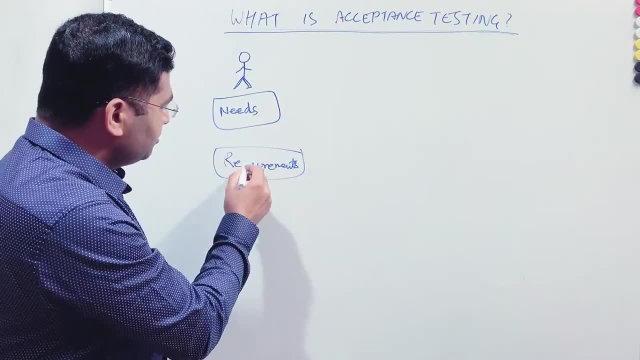 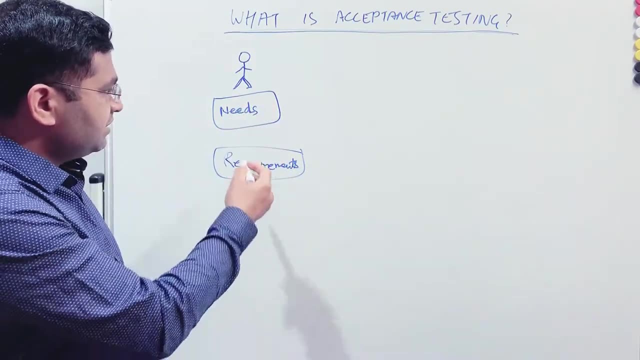 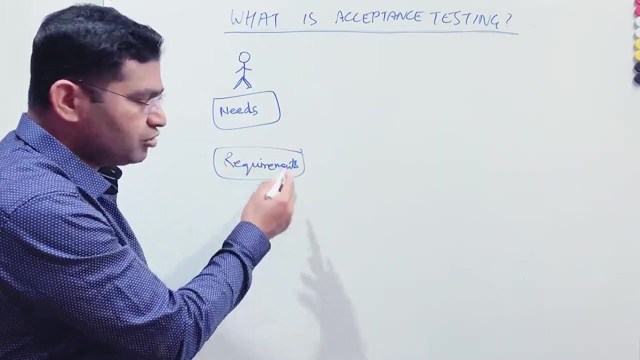 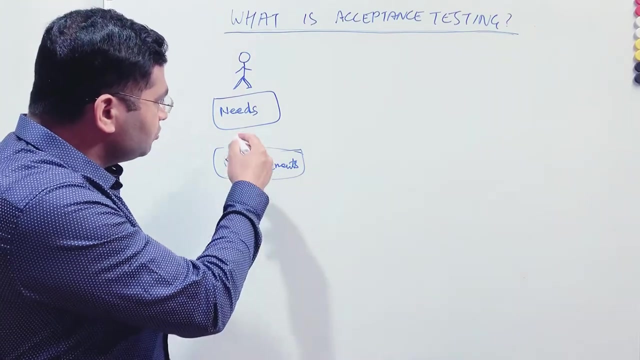 customer's needs be verified. so, for example, whatever he needed has been documented in requirements, but how does it mean that whatever he has wished for or needs has been clearly articulated into the requirement document or the user stories? right? so when that is the case? basically so in order to make sure that whatever requirements have been built throughout that. 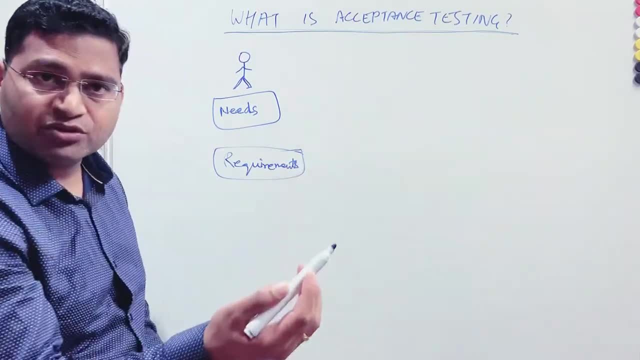 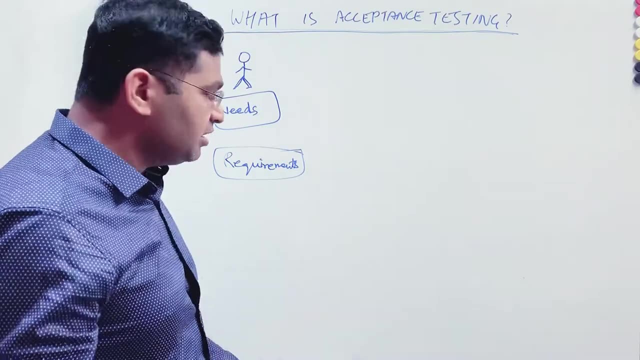 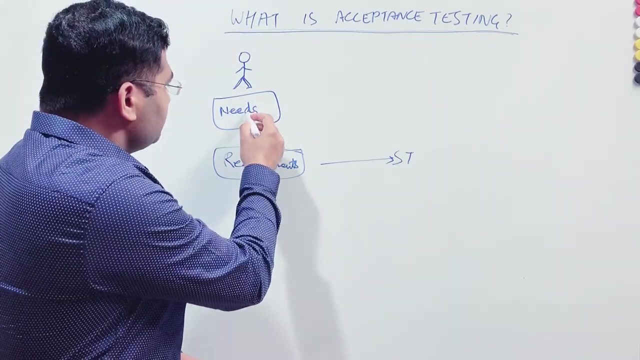 software development lifecycle and in the system testing we have anyways verified the requirement that, based on the requirement, the system is functioning fine, right, so that's what we have verified in system testing. okay, so in system testing that has been verified already now in order to verify the 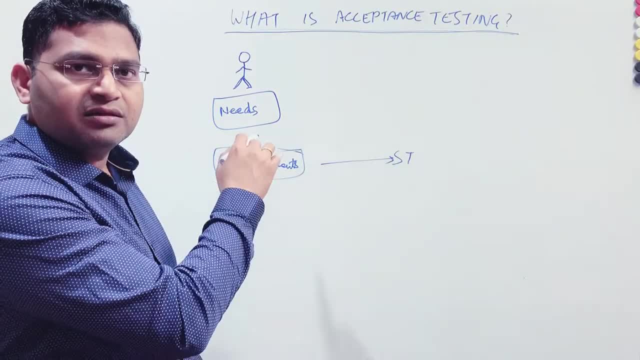 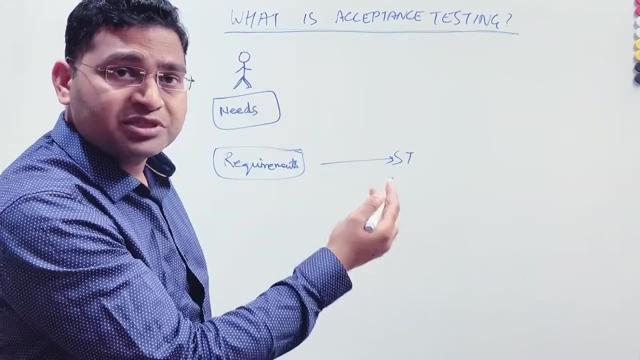 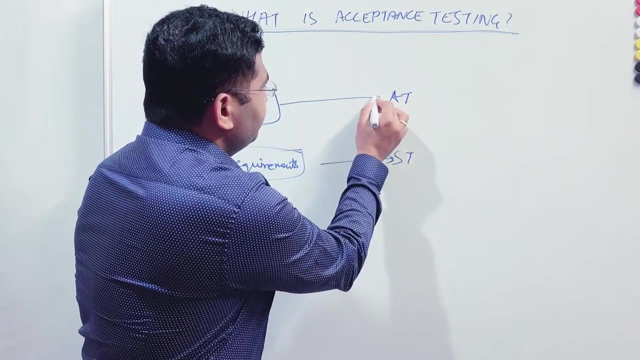 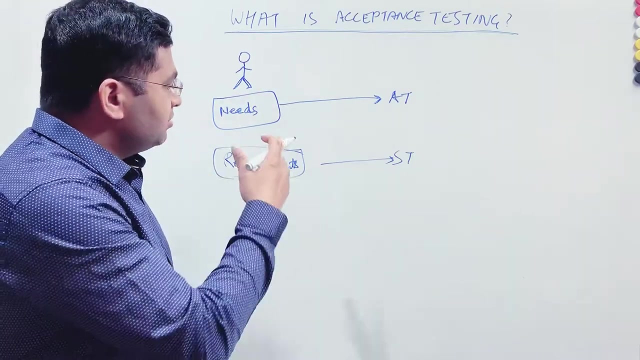 exact needs, or what the customer has you know initially, or what exactly he needs. user acceptance testing or acceptance testing comes in place. right, this is where your acceptance testing comes in place. okay, so what acceptance testing is all about is basically whether the software or the application that you have built, whether that. 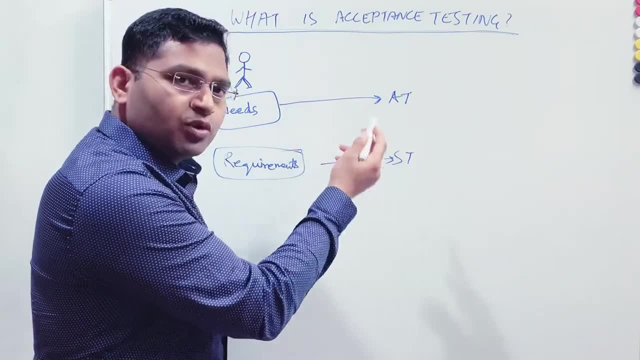 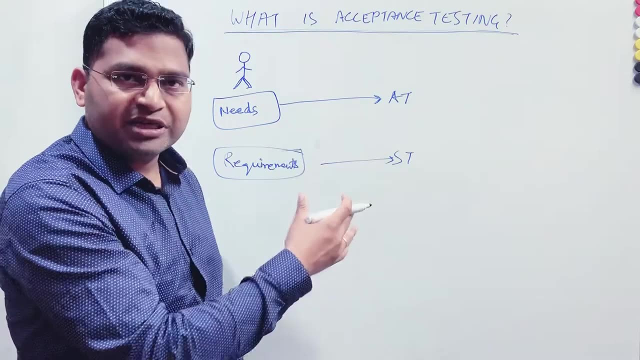 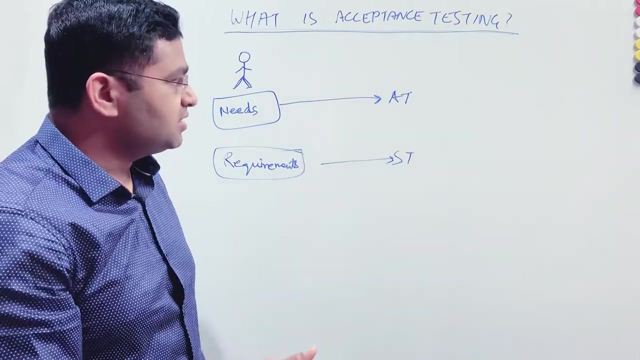 software fulfills the customer's requirement and it's fit for use or whatever customer needs. whether that software application fulfills that or not, is acceptance testing okay? now, there are many forms of acceptance testing, so you would have heard about the alpha test, alpha testing, beta testing, right? so alpha testing is. 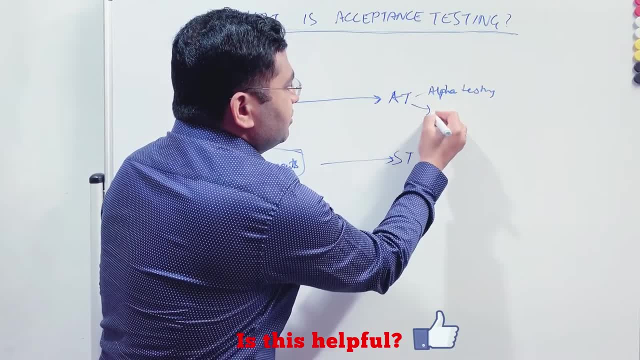 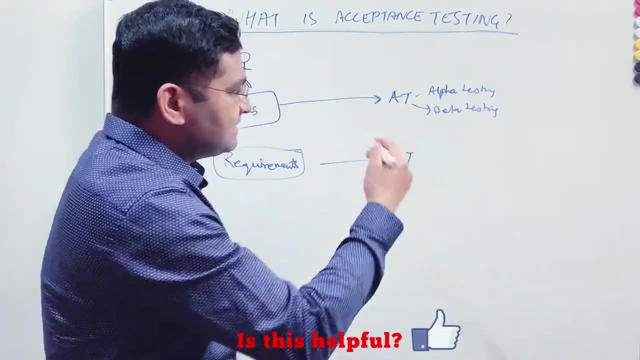 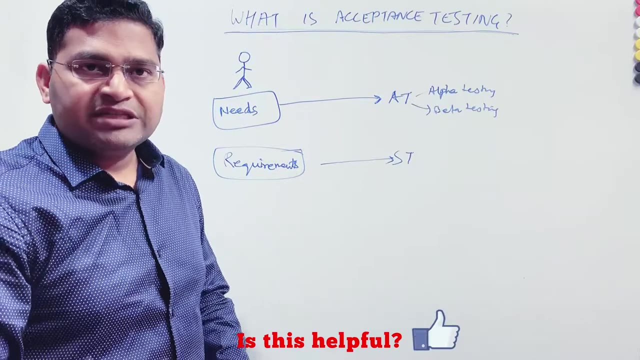 one of the acceptance testing: alpha testing, beta testing. now, what is the difference between alpha testing and beta testing? so in alpha testing, the testing is done at the development premise. okay, so wherever the development is happening within the development team, alpha testing is done. and most of the you know, like business stakeholders and other people. 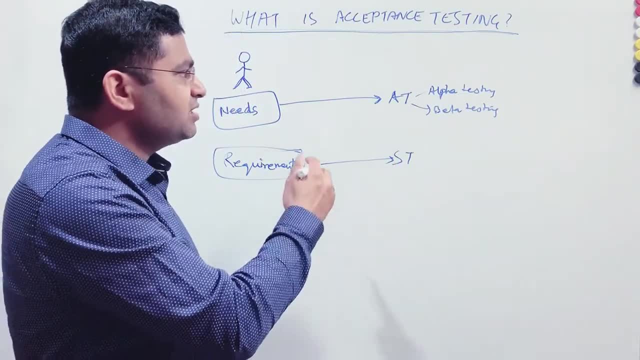 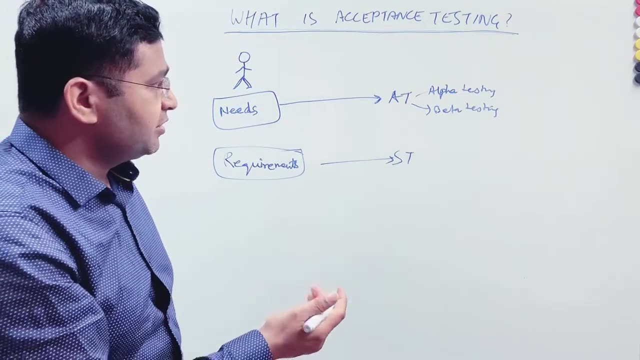 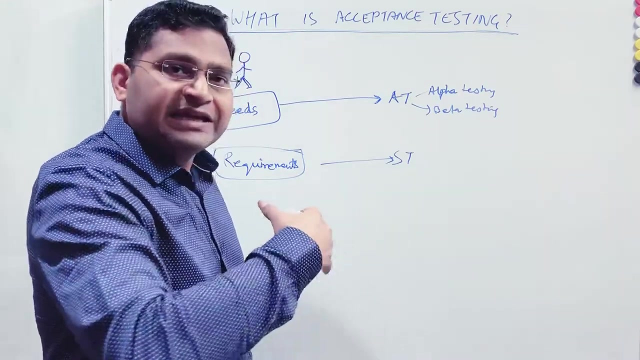 are invited to test the application and verify that the acceptance criteria has been met as per has been met as per the needs of the customer. beta testing happens at the other or the customer's premise most of the time, or the end user. so basically, if say, for example, we are testing a gmail, 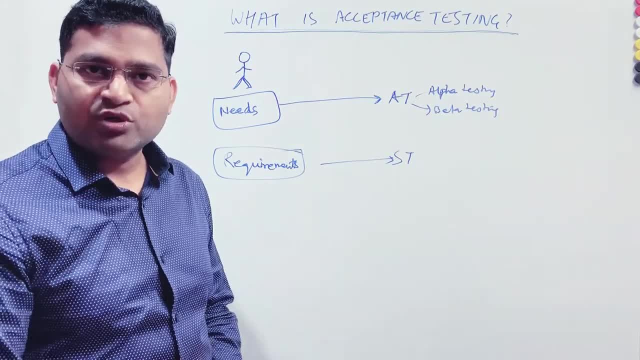 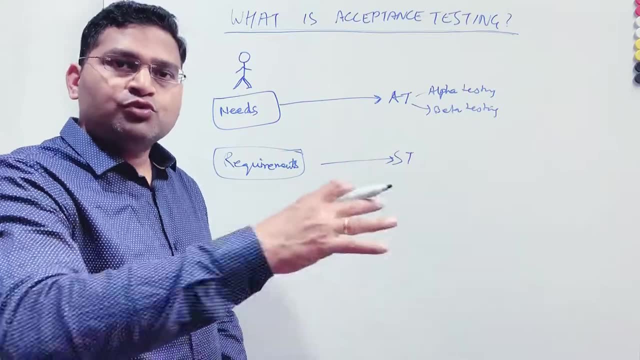 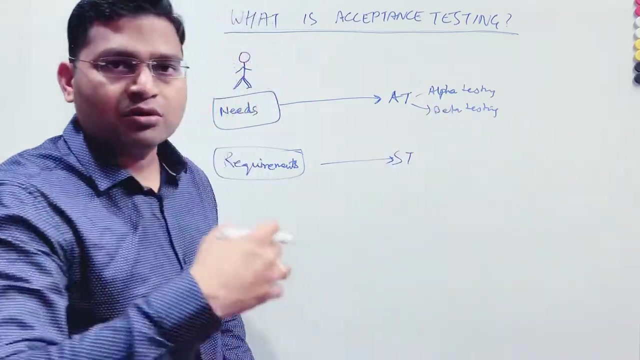 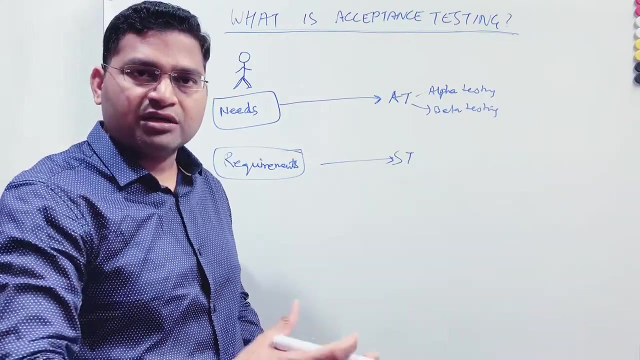 application, right, so gmail application, or these you know facebook application, these applications, you would have seen, sometimes the new features are being rolled out to few users or a section of users, so those, that is the beta testing. so, basically, what facebook does is, or all these you know applications or the softwares for which we are the users or end user, are the the people that 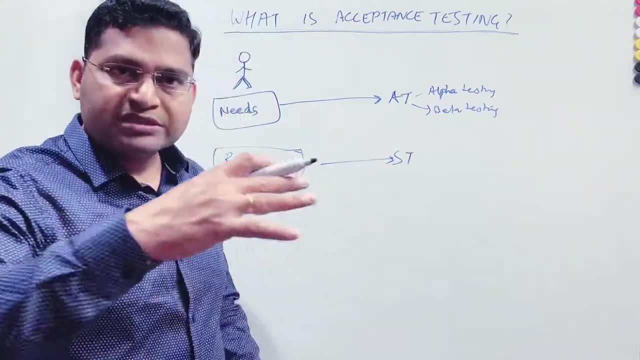 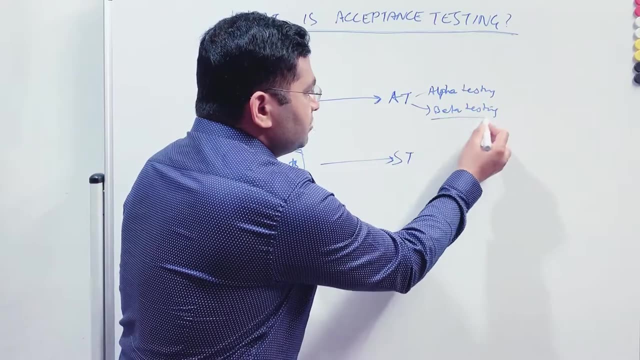 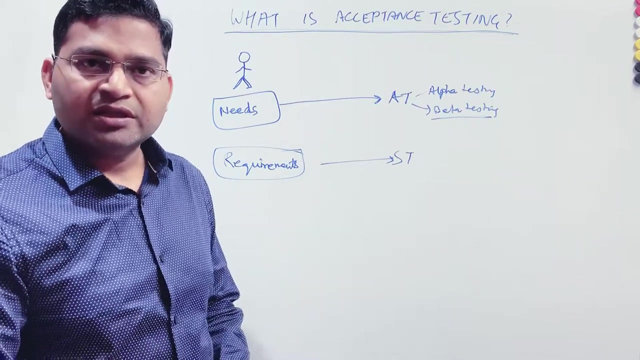 you know, use it day to day. then they roll it out to a set of users and those users use it and provide the feedback, and that is what beta testing is all about. right, alpha testing will be done internally at the google, you know, headquarters or google office with, with the help of business. 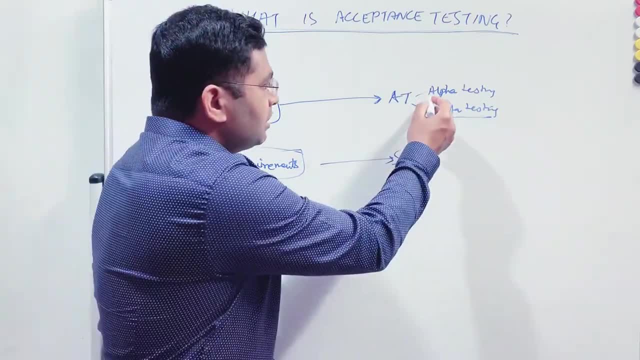 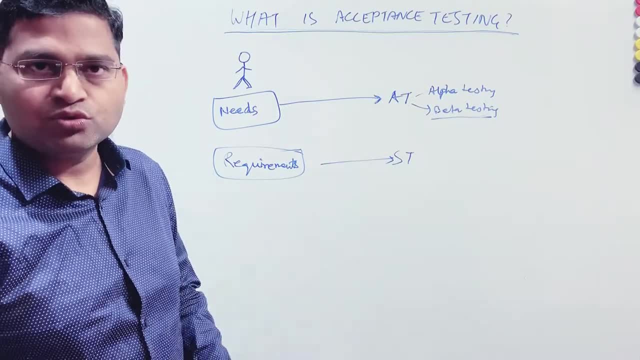 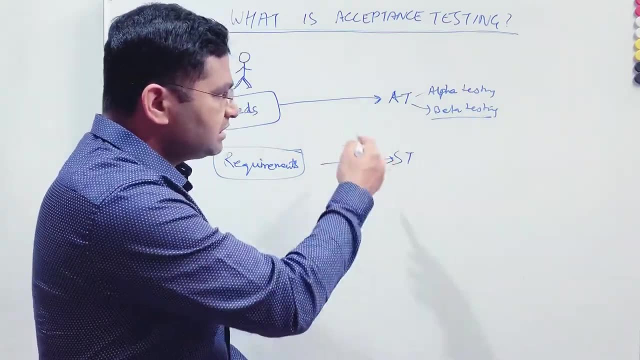 particular feature and report any issues if there are okay. so, as you use, if the software crashes, crashes, you will anyways report it to google, right? so that's what beta testing is. so this is. these are, you know, phases of acceptance testing. now there are many other type of acceptance.